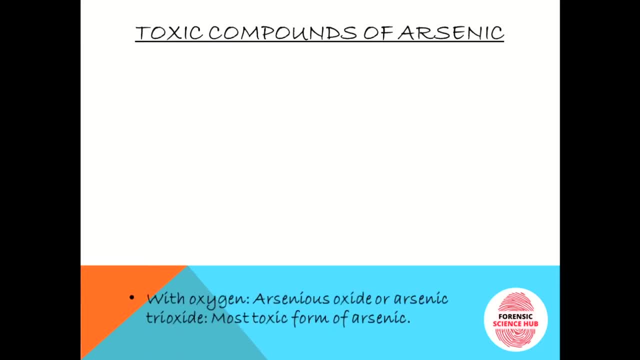 with oxygen, sulfur. So there are different compounds. First, with oxygen, arsenic oxide is formed, or which is also known as arsenic trioxide. Now, this is the most toxic form of arsenic. In common language, it is also called Sankhya or Somalkhar. This arsenic is white in color, So it 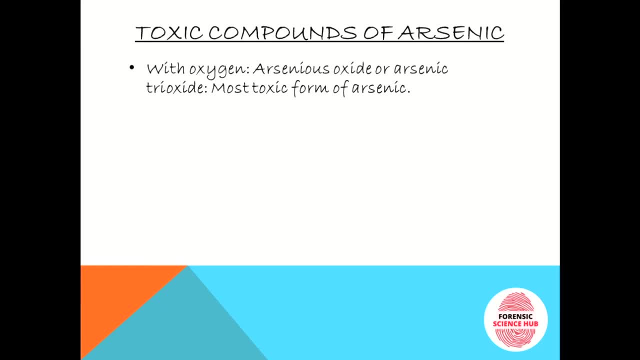 is also known as white arsenic. Now it has no taste, smell and is sparingly soluble in water. Then with copper it forms copper arsenide, also known as shells green. Another compound that is that it forms with copper is copper acetoarsenide, which 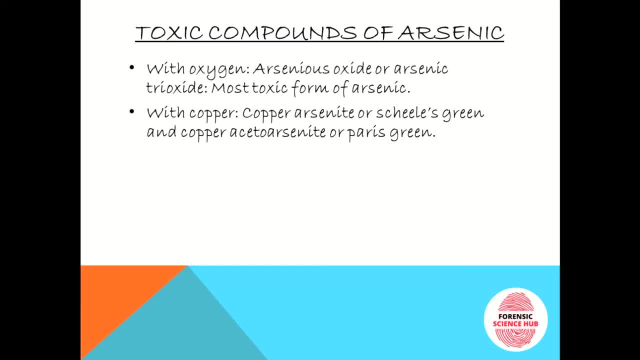 is also called Paris green or emerald green in color. Actually it is used in coloring agents for some substances, including confectionaries. Then comes with sulfur. With sulfur, arsenic forms arsenic trisulfide and arsenic disulfide. Arsenic trisulfide. 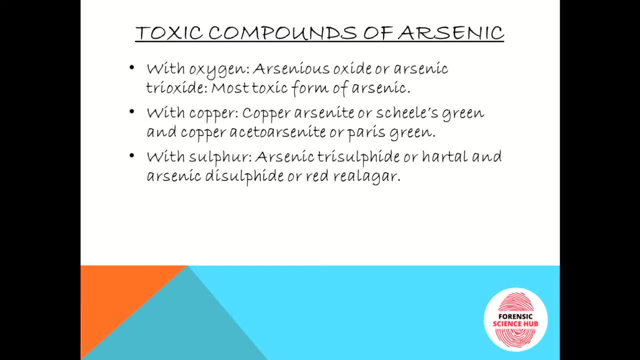 is also known as hartal or yellow orpiment, And arsenic disulfide is also called red realgar. Then red realgar is also used in as a coloring pigment in making flypaper. Then arsine gas. arsine gas is also quite poisonous. It is colorless and it has a garlic like 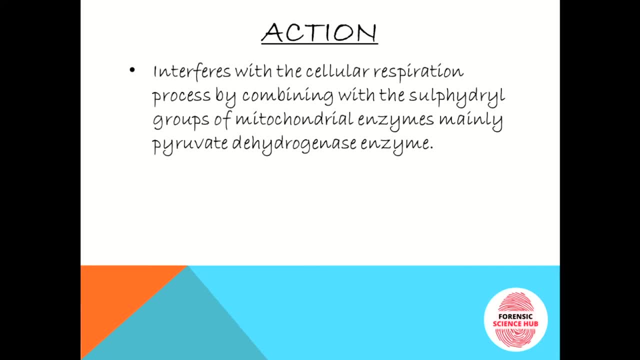 smell Now the action: How arsenic works when it enters our body. So it interferes with the cellular respiration process. So what happens is there is an enzyme called pyruvate dehydrogenase. This is a mitochondrial enzyme. This enzyme, 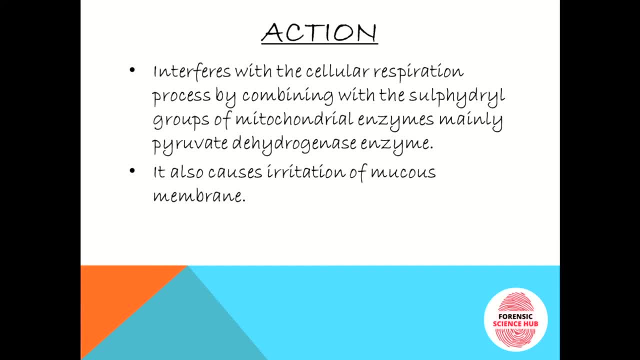 is responsible for a reaction that converts pyruvate into acetyl coenzyme A from aspartic acid and lumière. But this enzyme is responsible for a reaction that converts pyruvate into acetyl coenzyme A and pyruvate as a modification Aldições, And the reason is because it is committed for rodz immerter L родen. 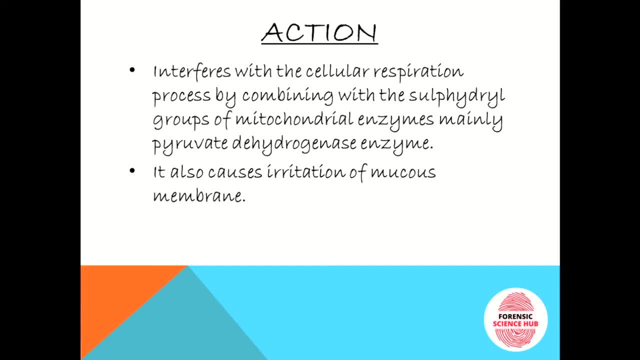 It is remarkable. we don't know even how, or if you realize this, then we don't know about the usage of this enzyme. you know, the product of glycolysis cycle is pyruvate and it further has to be converted into acetyl coenzyme a. now this enzyme the arsenic. basically, it binds with the self-hydrile groups of. 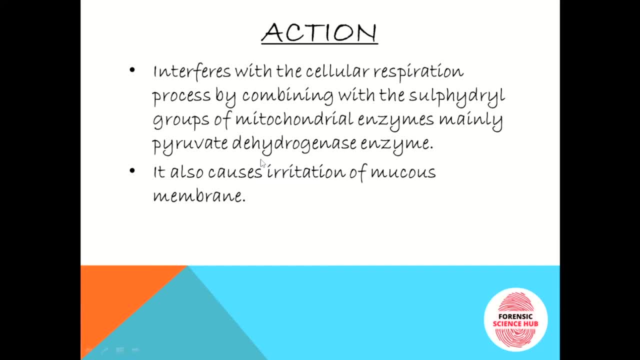 this enzyme, pyruvate dehydrogenase. so therefore this reaction doesn't occur and that's how it interferes with the cellular respiration process. also it causes irritation of the mucous membrane. also it is carcinogenic substance. now let's talk about the acute poisoning. you know poisoning are. 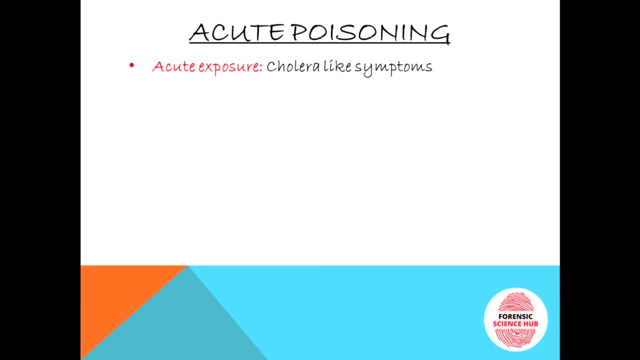 of two type: acute and chronic. acute means large amount of poison, irritant whatever, has been taken at the same time and which causes a series of problems. and in chronic poisoning small, small amount is taken for a very long time. so for for discuss acute poisoning. in acute poisoning it is further of two types, so acute exposure here. 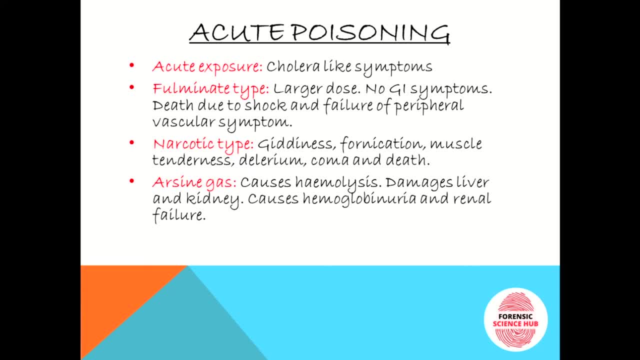 cholera like symptoms can be seen. there is throat constriction, intense thirst, difficulty in swallowing the stool is involuntary and it is frequent, and first it is dark, bloody in color, then it becomes colorless, odorless rice water like so. this is if these types of condition are seen. 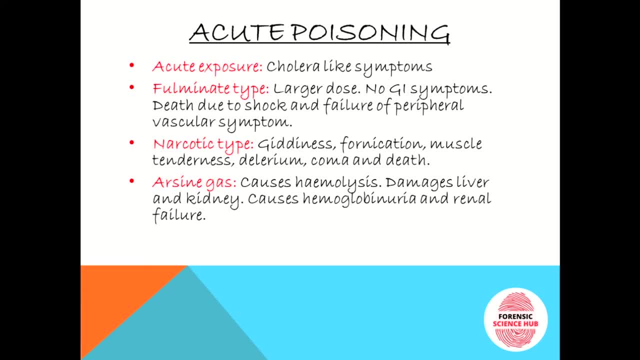 then we can tell that this is a acute exposure of arsenic case, then fulminate type. now if more than three grams of arsenic is taken, then we call it fulminate type. in this there are no gastro intestinal symptoms seen in acute poisoning. i forgot to mention that there are gastrointestinal symptoms and also in acute 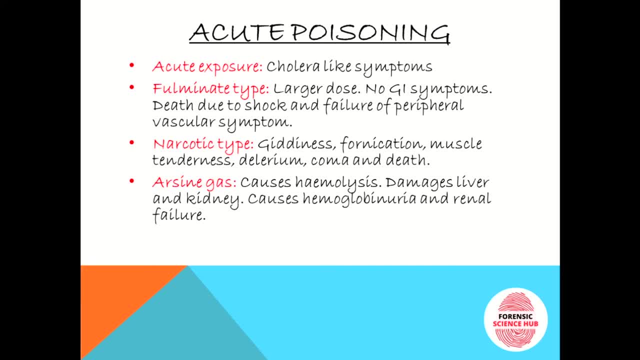 it is very important to remember that it causes cholera-like symptoms. so in question sometimes can be asked which of the following irritant has or shows cholera-like symptoms. so the answer will be arsenic coming back to fulminate. um, there are. here are no gastrointestinal symptoms, but here. 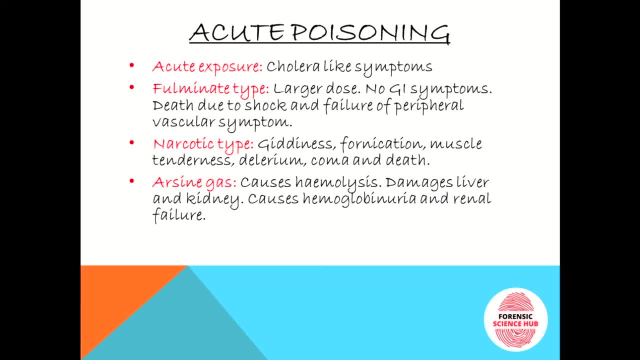 death occurs due to shock and failure of the peripheral vascular system. there is a mistake, its system then. third type is narcotic type. here, giddiness, fornication, muscle tenderness, delirium, coma, death, all these are the symptoms. fourth, arsine gas. it causes hemolysis, it damages the liver and kidney. basically, arsine gas. 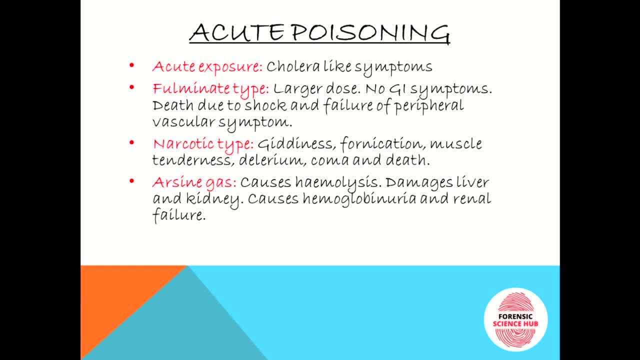 is a vapor form of arsine. okay, this is formed when arsine combines with hydrogen and arsineurated hydrogen gas or arsine gas is produced. it causes hemoglobinuria. hemoglobinuria means hemoglobin is found in the urine of the person and renal failure. here a black color urine is found if there is hemoglobinuria. 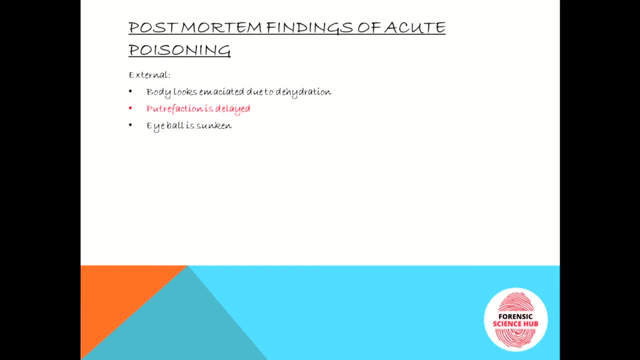 then the post-mortem findings of acute poison. the external appearances looks like the body looks emaciated due to dehydration. uh, putrification is delayed. this is important point. then eyeballs are sunken internally. if we see the mucous membrane of mouth farrings and esophagus nature inflammation. 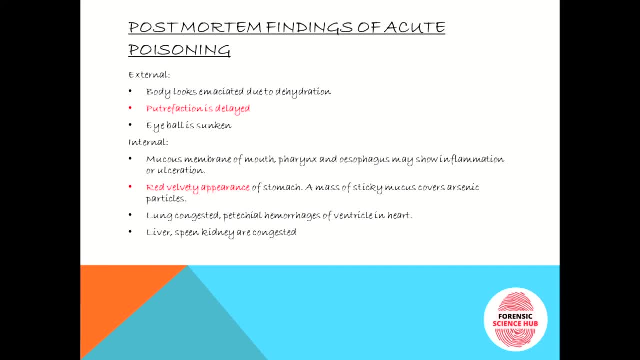 now. another important point is red, velvety appearance of stomach is seen in arsenic poisoning cases. a mass of sticky mucus covers the arsenic particles. Lungs are congested. Particular hemorrhages are seen in the ventricle of the heart. liver, spleen, kidney are congested. Then chronic poisoning. Now there are six. 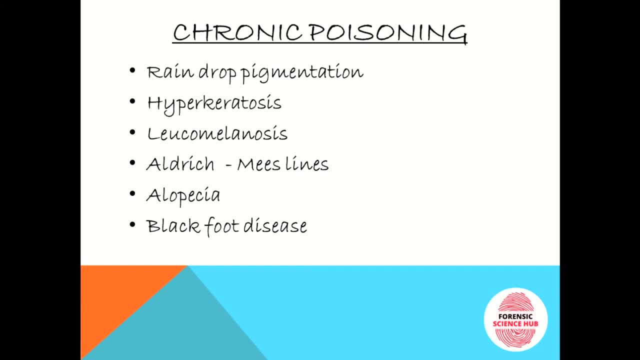 different and important symptoms that are seen during the chronic poisoning. First is the raindrop pigmentation. Here brown color pigmentation is seen on the skin and shoulder. So since there are drops seen, it is known as raindrop pigmentation. Next comes hyperkeratosis. 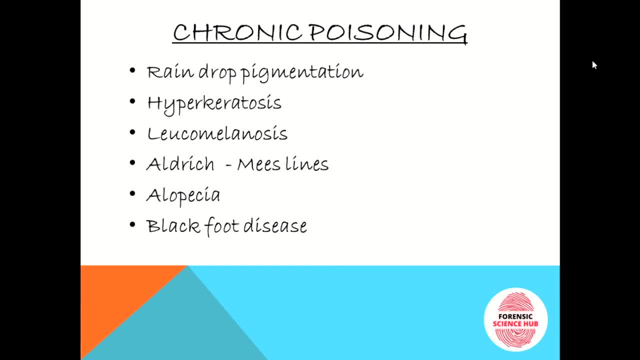 In hyperkeratosis there is increased amount of keratin that is deposited. So because of that, it is deposited on the nails. Okay. so because of that, there is excessive irregular thickening of the nails. Next is leucomelanosis. Now in this, there. 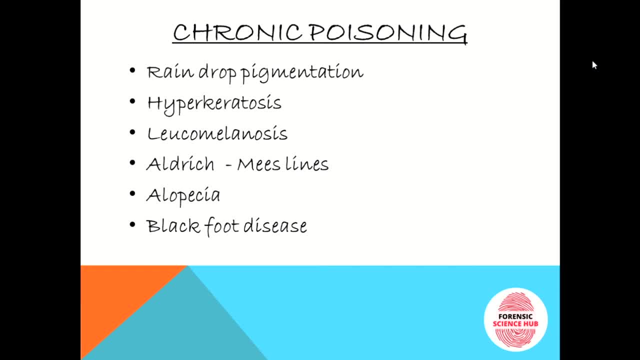 the macular areas of depigmentation may appear on the hyperpigmented skin areas. You know leucomelanosis, melanin. Melanin is the pigment that gives color. Okay, so in this there is hyperpigmentation. There are more amount of melanin is deposited on the body. Next important: 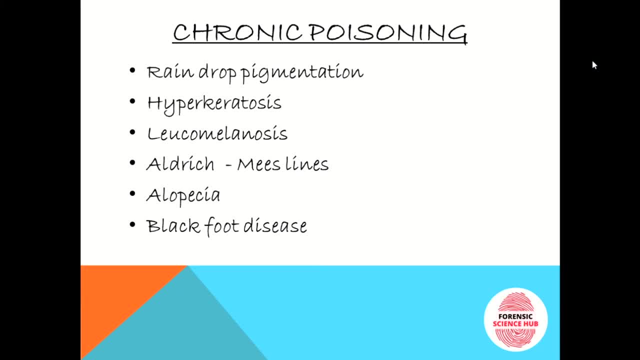 thing is Albrecht Mies lines: These are basically opiates, These are basically opiates, So these are basically opiates, So these are basically opiates, So these are basically ornithologist. These are basically, which are mainly white bands that are formed on. 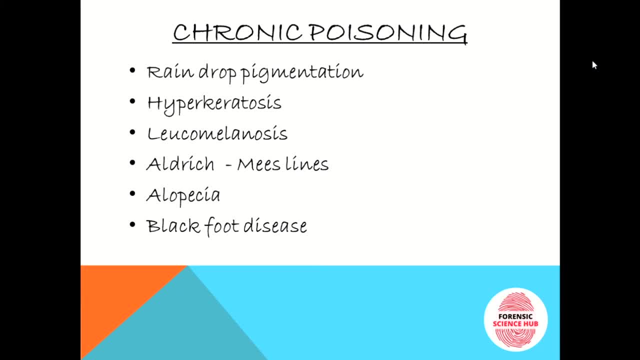 the nails of the finger and the toes. This is very important. Then comes alopecia. This is basically here. follicles in this are affected. Last but not the least, Blackfoot disease, in which the peripheral vascular- it is a peripheral vascular disease- that is characterized. 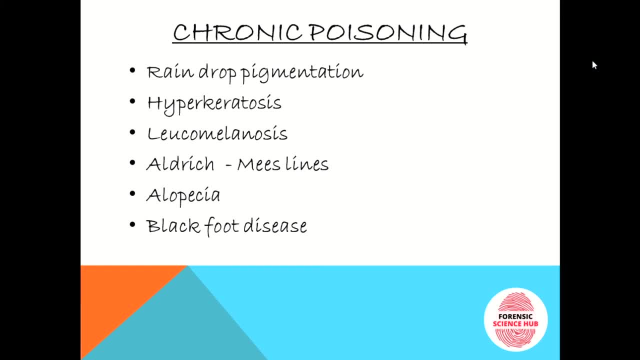 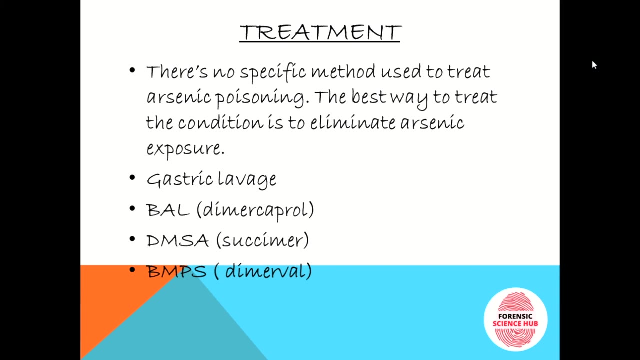 by systemic arteriosclerosis. In the next slide let us see the side effects of Albrecht Mies lines. Now, after we have so in this, the post-mortem findings is that the fatty yellow liver can be seen. now treatment is no specific treatment, the best way or the most important thing that one needs to. 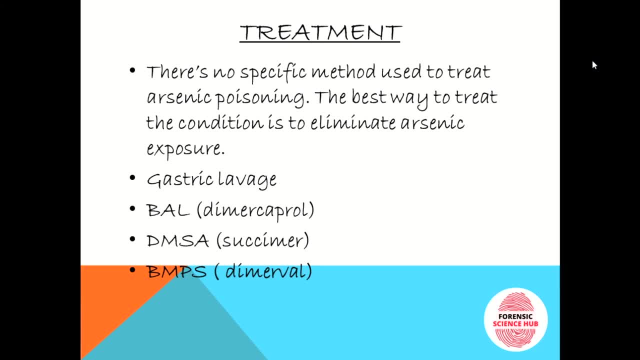 do is eliminate the exposure. okay, so remove the source of arsenic. then comes the gastric lavage. it is done repeatedly with large amount of warm water and milk. activated charcoal does not absorb arsenic and it is not, hence not recommended. then there is an important antidote, which is 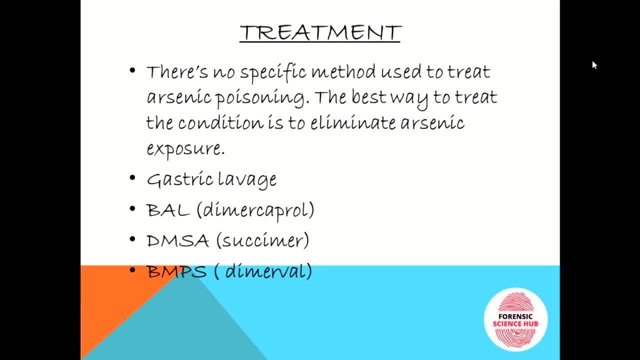 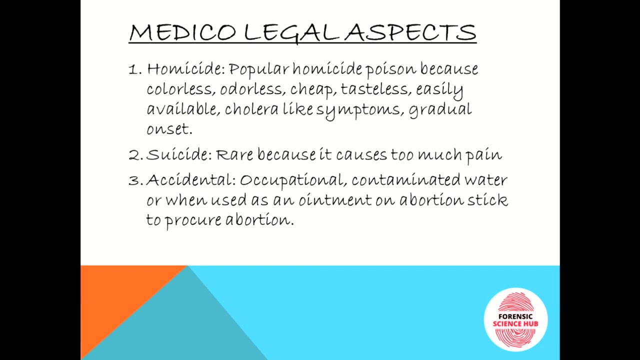 bal or b-a-l. it is also known as dimer caprol. another important antidote is dmsa or succimer, and also dm bmp- sorry, it's dmps or dimer wall. now the medical legal aspects. uh, first, if homicide, then it is a very 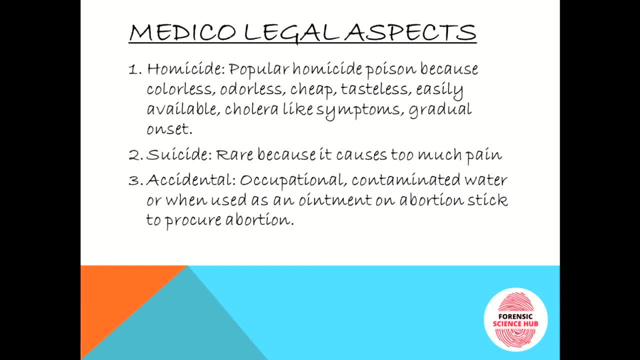 popular homicide poison, the reason being: it is colorless, you can drink it, you can mix it in any drink for whatever, and not that i'm saying that you should do it. uh, and it is odorless, so no one comes to know about it. cheap, easily available, tasteless, 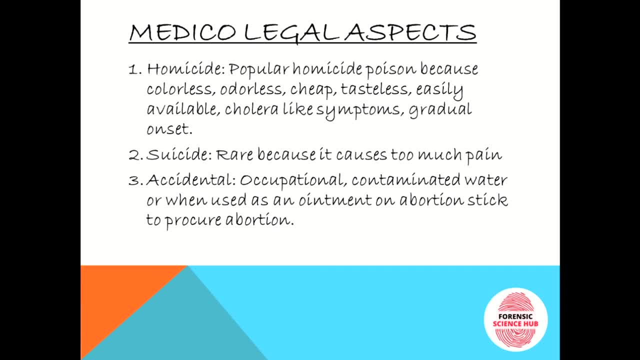 it has cholera like symptoms, so the person won't even be able to detect and it it's gradual onset. so people uh generally won't come to know right in the start that they have been poisoned. then for suicide it is not generally used because it causes a lot of pain then accidental it can be.